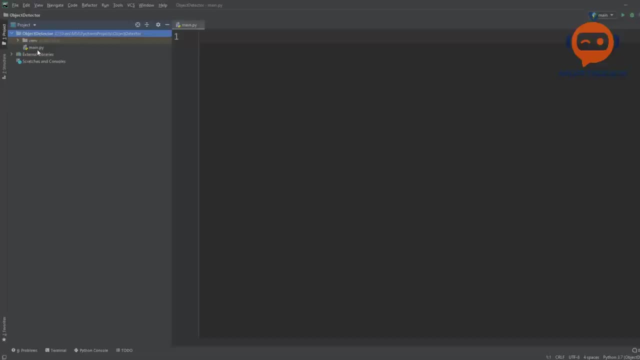 this object detector project And inside that we have a main dot py file. Now we are going to write all of our code in this mainpy file. Now, before we start, we are going to import a few things. So we are going to import a few things. One of the things that we are going to import is the 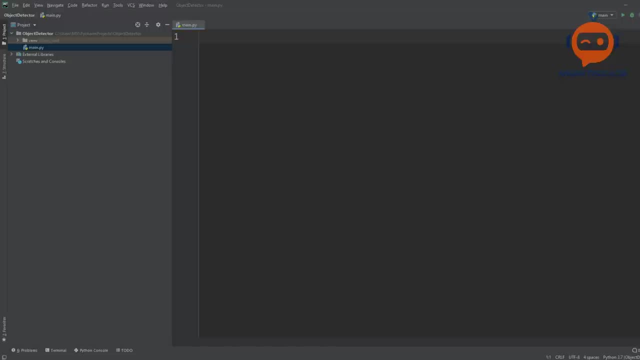 so the first one is basically our image, and then we have the coco names. let's copy these. so here we have the coco names. so these are the- what do you call- classes that we can detect. so we have person, bicycle, car. so if you want to know more about this data, you can. 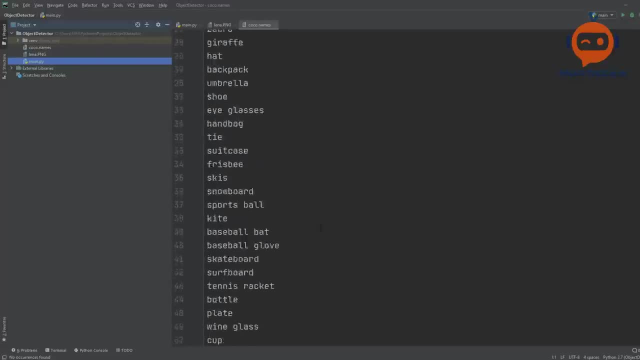 check the coco data set. this is very common and very popular. so- and this is our image, lenapng. so we will detect the face on this and then, once we do that, we are going to run it with our webcam. and what else do we need? we need the weights and configuration file. 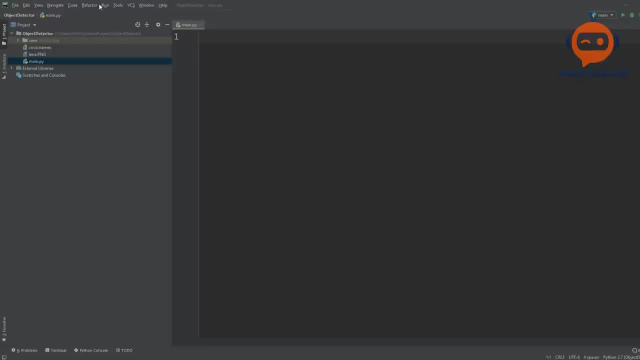 so, basically, what we are using is the mobile ssd and we are going to import its files. now, you can see, here we have, uh, these are the latest files. you can see that. uh, it shows uh. okay, this one is the old one, it's 2017. i will delete that. where is the other one? 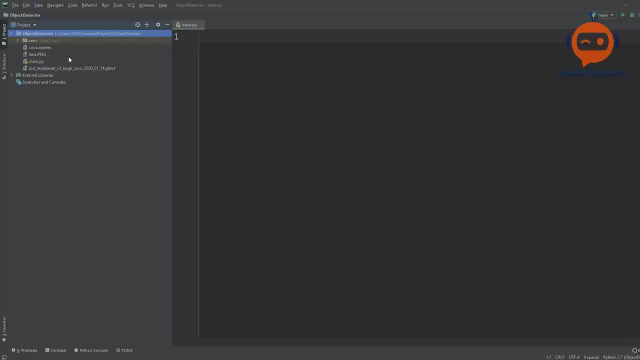 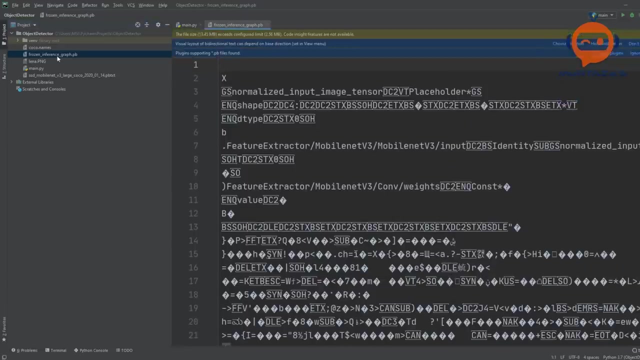 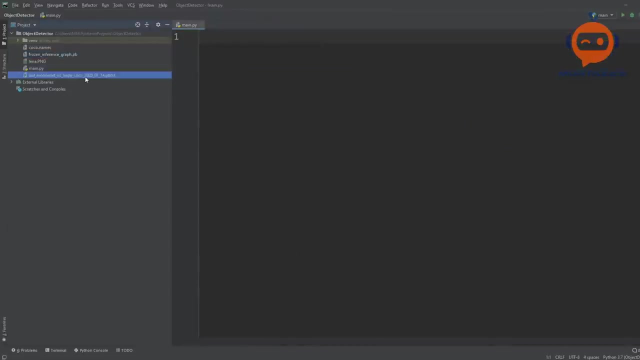 uh, okay, this is the actual weights. did it copy? yes, okay, so these are the weights. and, uh, of course, when you open this, it will be gibberish, so we'll just close it. and then we have the architecture, or the configuration, so we have all the information over here. 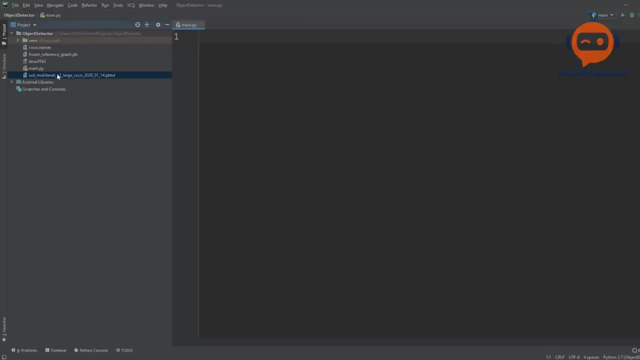 and we can close that as well. so these have a little bit of a lengthy name, but i guess it's fine. so this is, uh, the latest update, which is version three, and you can see it was in 2020.. so in the beginning of 2020 this was released, so these are basically available on the OpenCV. 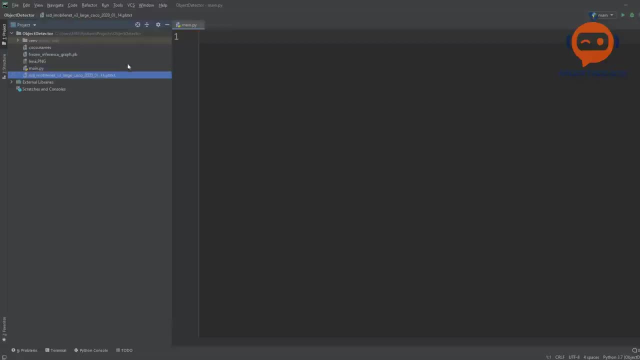 documentation, so i have downloaded it from there. so i will put a link to these files in the description so you can download them as well. so the reason we are using the MobileNet ssd is because it is one of the best methods right now which has a good balance between accuracy and 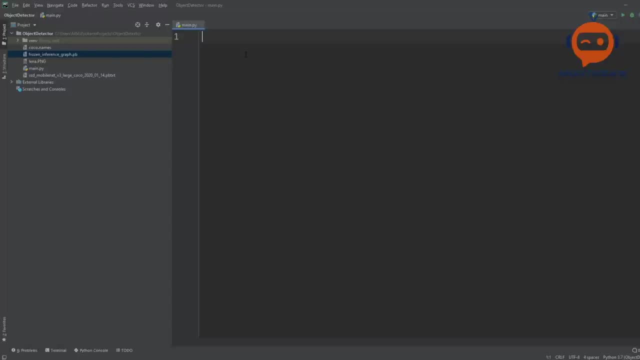 speed so we will be able to run it at the moment. this is the one that we are going to use in the future, so we will see with our CPU almost real time, and it will be able to detect a lot of objects with a good amount of accuracy. now, with Yolo, we have to use GPU, otherwise it's. 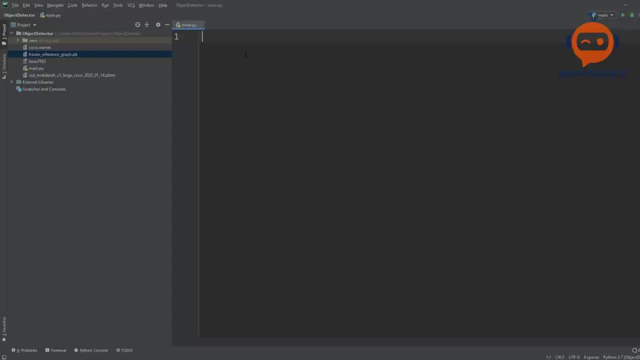 too slow and if we go for the Yolo tiny it's not that good. so if you are trying to detect some objects, some common objects, it's not that good if you use Yolo tiny. so mobile net SSD can be used with Raspberry Pi and Jetson nano as. 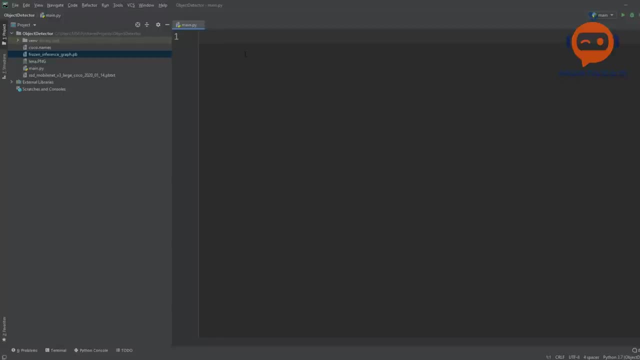 well, because it is lightweight and you can get a decent amount of accuracy. so this is the reason that we have chosen this, and this is the latest update, so I'm hoping that it will be better than before. so let's get started with that, and now that we have all the files that we need, we will go to files settings. 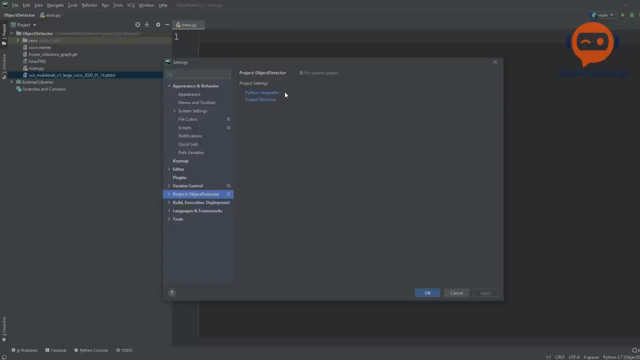 and then we will download, I will go to the interpreter and we will install open CV. so this is the only library that we need. so we will write here: open CV Python by turn, and there you go. so we will install this. okay, so now that the installation is done, we will close it and over here we are going to write. 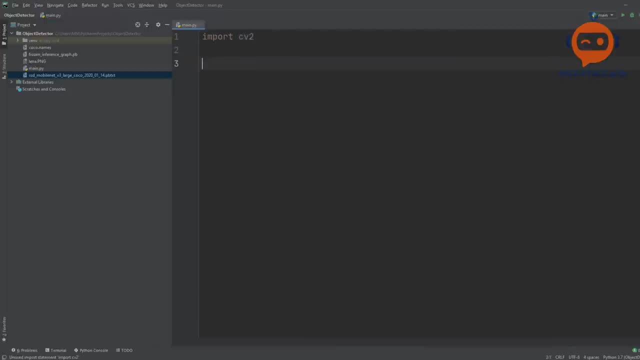 import cv2. so the first thing we need to do is we need to import our image. so we are going to say that our image is equals to CV2 dot. I am read and we want to read lineup so Lina, not PNG, that is correct. and then we can simply display. 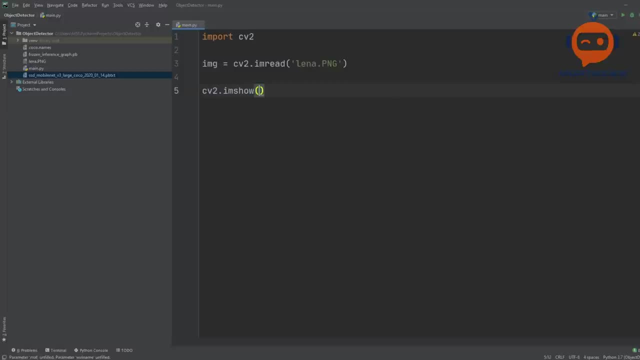 this. so CV2 dot- I am show. let's say how to put. and then we can say: import cv2 dot- I am show. and then I'm gonna print out to the going to import cv2 dot- I am read and then we can simply display this. so cv2 dot- I am show. let's say output and then 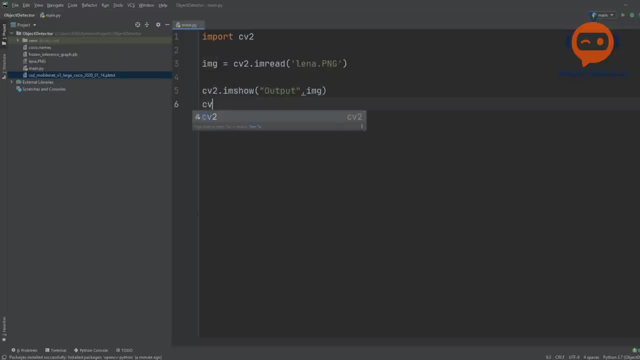 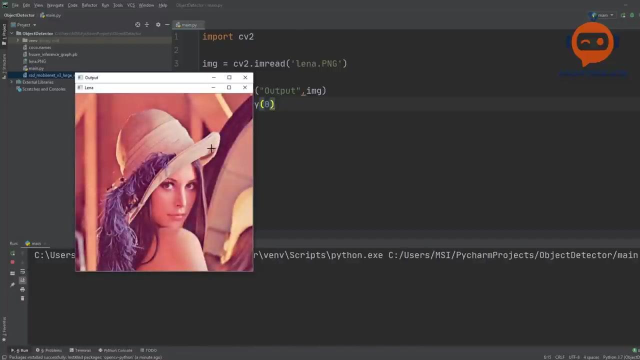 we will say that we want to display our image, and then we can write cv2 dot weight key- cv2 dot weight key, and let's put zero, okay, so let's right click and run this and there we have it. so now we can see that we have our image now, okay. 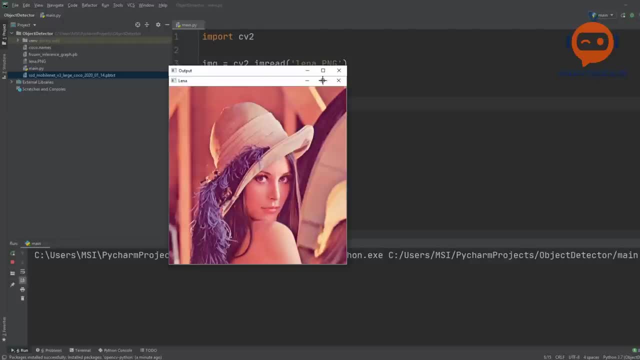 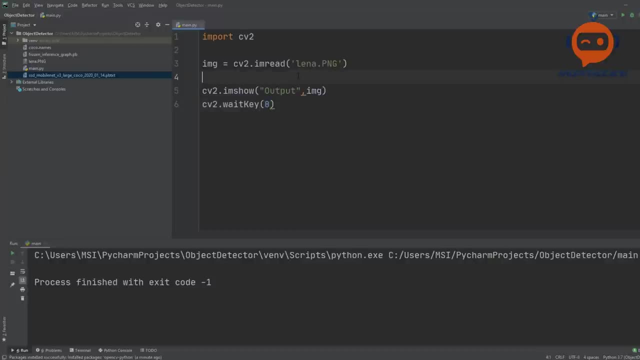 I have copied the wrong image. actually it has this anyways. it shouldn't matter that much, okay? so once we are done with that, we are going to first import our names of the cocoa data set. so the thing is that these are a lot of names, so you. 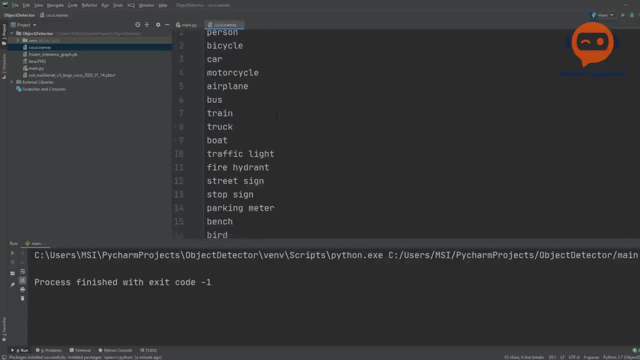 can see here we have a total of 91 names, so I'm going to import it automatically rather than importing or writing it down manually. so you can do this, so you can actually write, for example, class names. and you can write, for example, we have person, then we have car, and then we have. 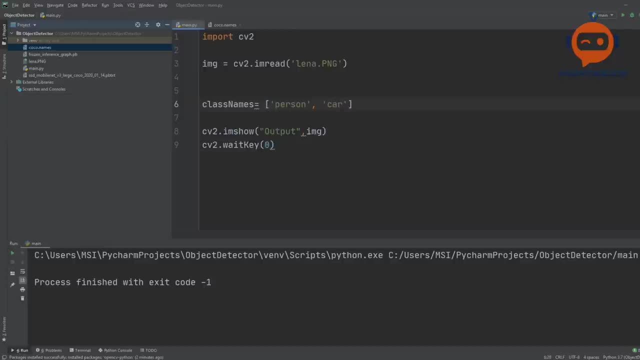 like this car, etc. etc. right so, but this is a bad way to do it, because we have 90 different classes and it's not going to work. it will be too lengthy to do so what we will do is we will simply import it. and to do that, we are going to say: 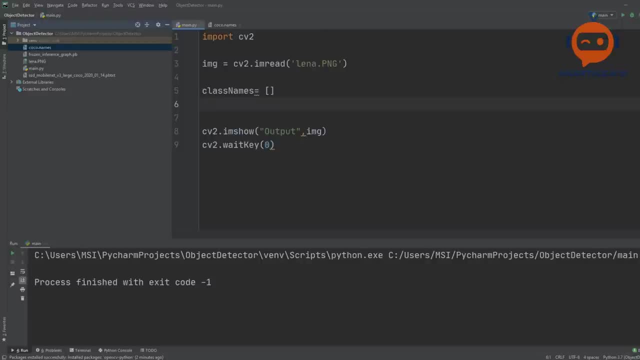 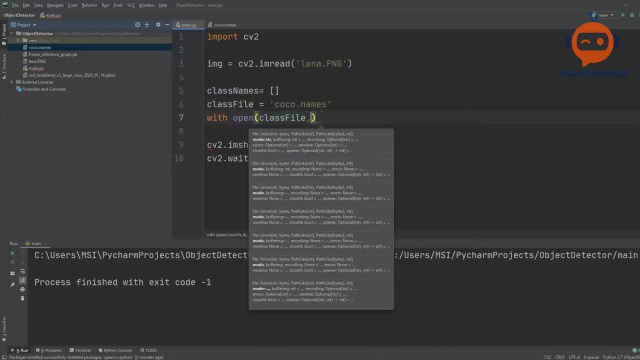 that our file, basically our class file, is our coco dot names, and then we are going to use with open to actually open our file, and we will say that class file and we want to read it, let me write it like this: and then we are going to say as F, then we are going to write our class names, which is this empty matrix or array, and then 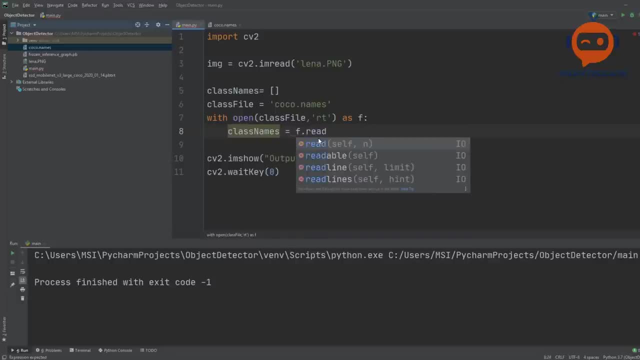 we are going to write that F dot read and we will write dot strip our strip. and then we are going to strip it based on a new line, and then we are going to write that we want to split it as well, again based on a new line. so this, basically, what it does is it puts all of this into class names. 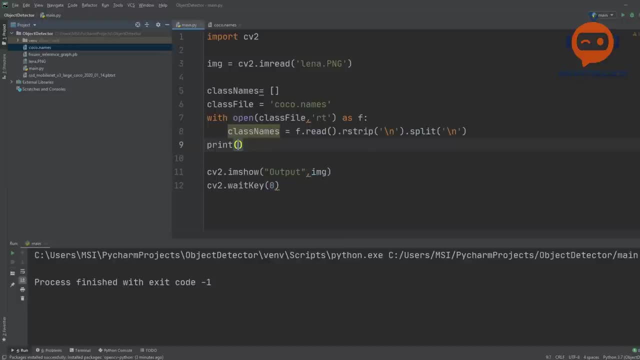 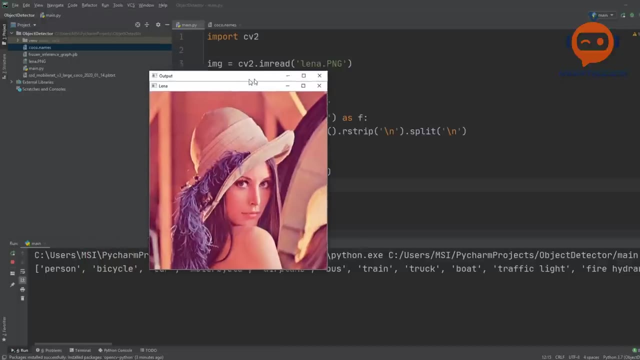 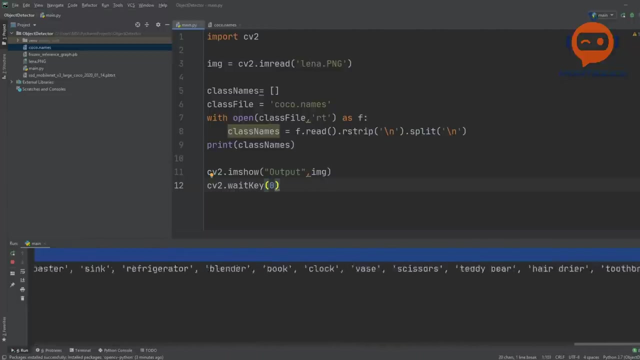 and let me, let me print it out so you can see. so prints class names and let's run that and there you go. so now you can see we have person, bicycle, car, motorcycle, so all of them in one single list. okay, so that is good. and now what we will do is we will import our files. so the first thing we have to import, 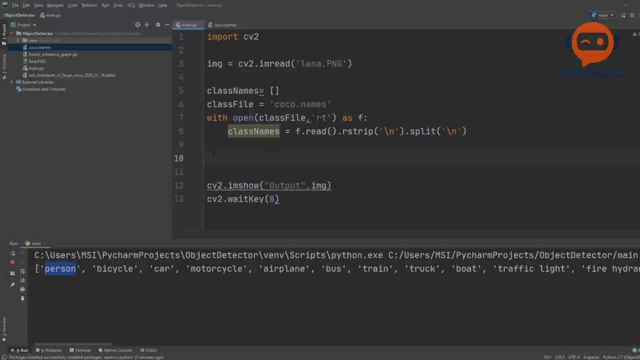 is our configuration file, so we will write here the path, because the path is a little bit lengthy, so we are going to write it like this. so we will write config. path is equals to. we will write down the name of this. so what we can do is we can double click this, we can right click. 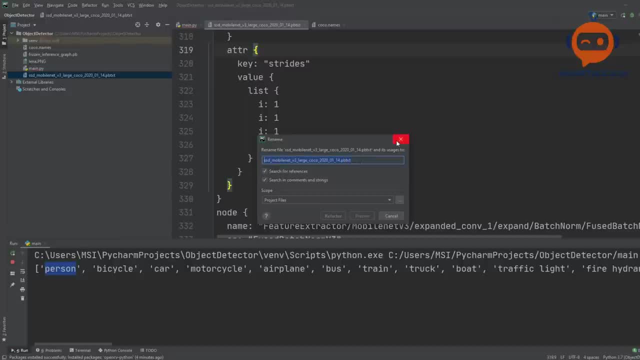 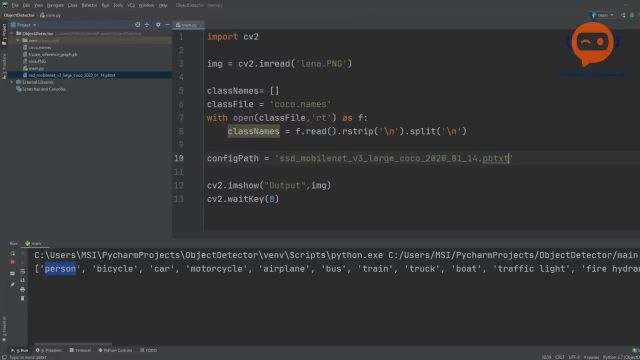 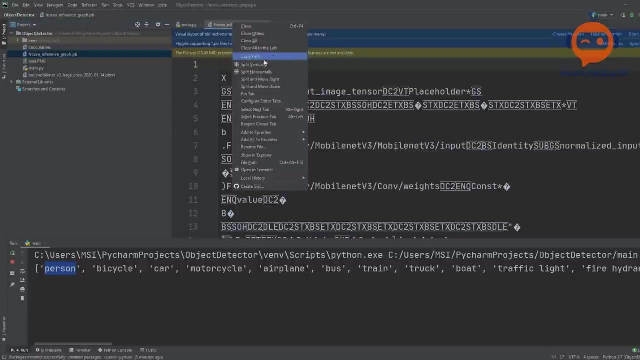 and we can write rename, and we can copy all of this instead of writing it down- I know it's lazy, but you know what, sometimes it's good to be lazy- and then we will write the weights- so weights path- and we will write here again. we can do the same thing. we can double click that, right click rename and we 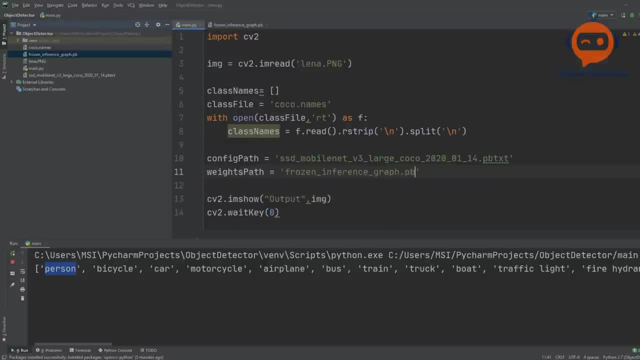 will copy all of this and we will paste this. okay, so both of them are now good to go. now we can simply create our model. so the good thing about OpenCV is that it already provides us with a function that actually does all the processing for us, and all we have to do is we have to input our configuration, path and weights. 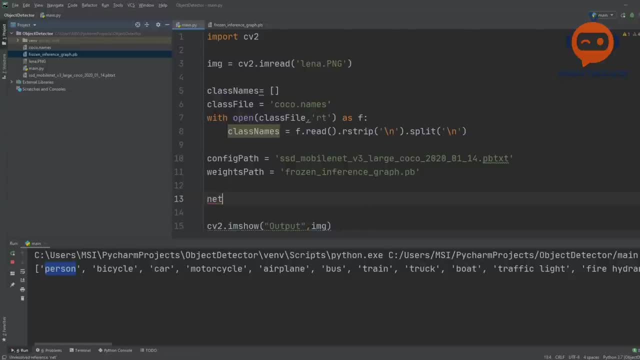 path and that's it. so if you have seen my Yolo video, it was a little bit different, where, after passing what do you call our image to our net, we had to apply some techniques to actually extract the bounding box and everything. but in this case it's very simple. all you have to do is you have to pass the image. 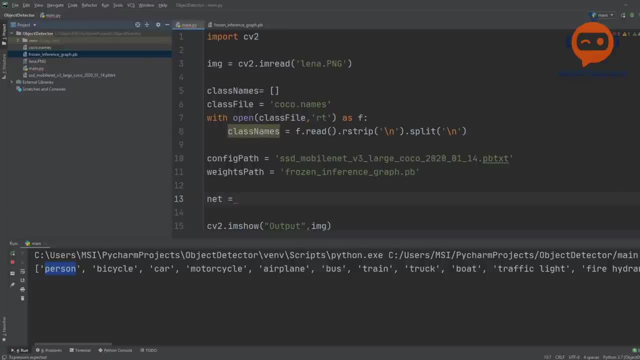 and it will do everything for you and at the end you will get a bounding box and you will get the names of the IDs. actually, you will not get the names, you will get the IDs and from IDs we can get the names of the objects detected. so here we are going to write: cv2 dot. 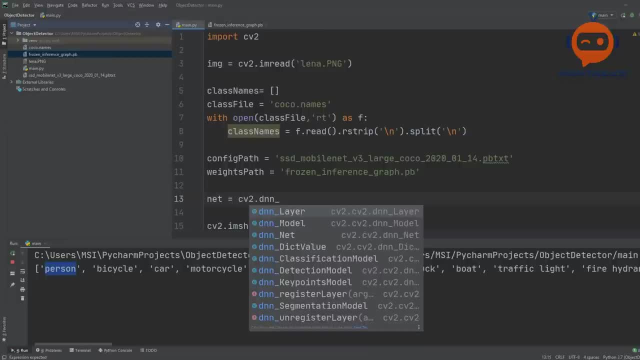 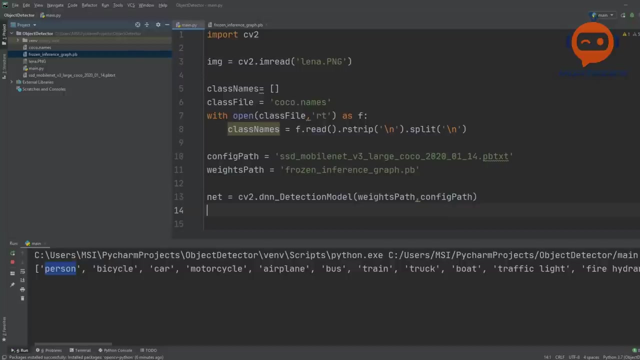 what do you write? dnn? underscore: detect model: detection model. yes, so we are going to give in our weights path and then we will give in our configuration path. so that is good. and then we have a few parameters that are set by default and I'm not going to play around with those. these are: 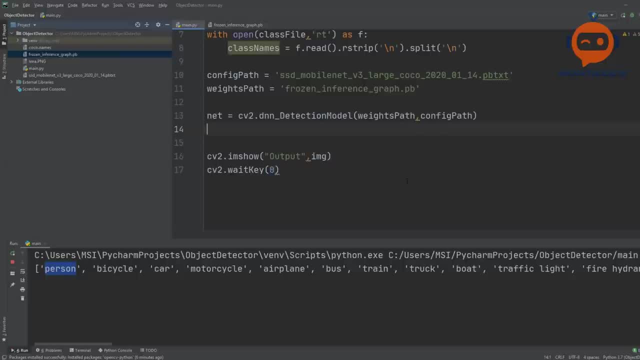 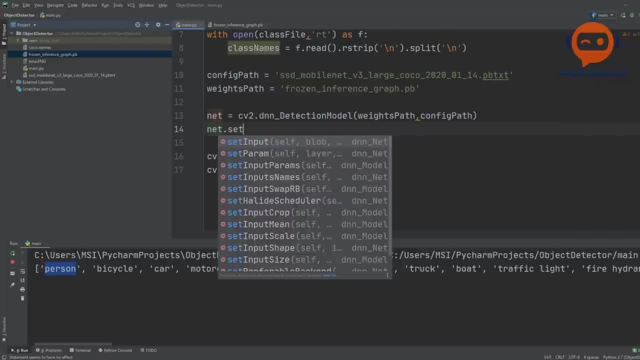 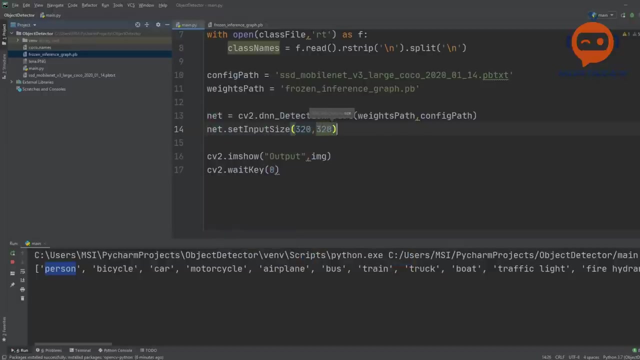 the configurations that I found on the documentation and we are going to use the same ones, so I will just write them down. so the first one: we have the input size. so input, where is the size? yeah, input size, and that should be 320 by 320.. then we have net dot set input scale, input scale and we are going to write: 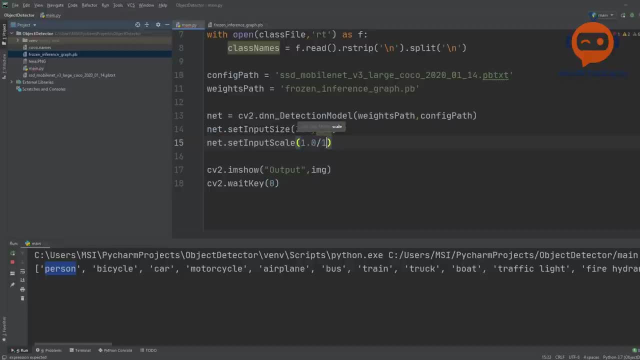 1.0 divided by 127.5. let's give a little bit space and then we have what? do we have the mean? so net dot sets input and we are going to write the mean, mean and then we have the values as 127.5 and then 127.5. 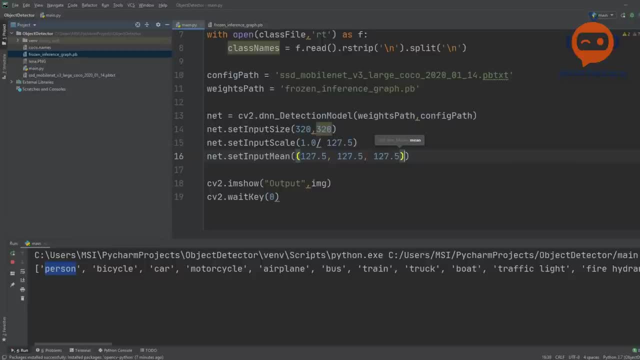 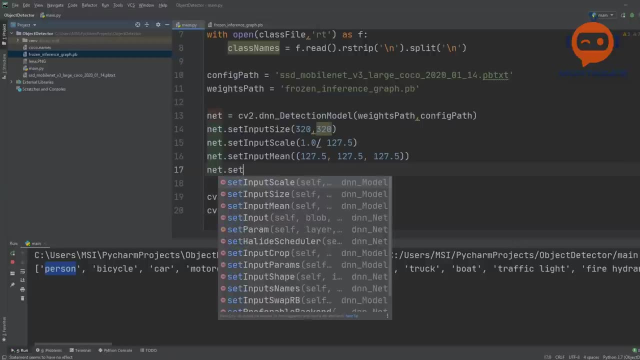 and then 127.5. so again, you don't have to worry about all these values. just follow along and think of this as something that is required to run. so later on, when we are doing another tutorial where we are using our own data to train our model, then we will look into the details and I will explain everything. what this? 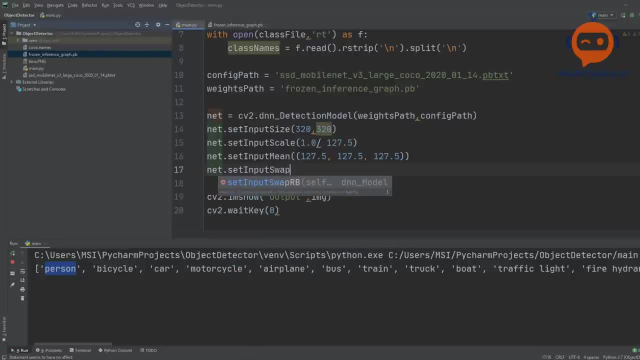 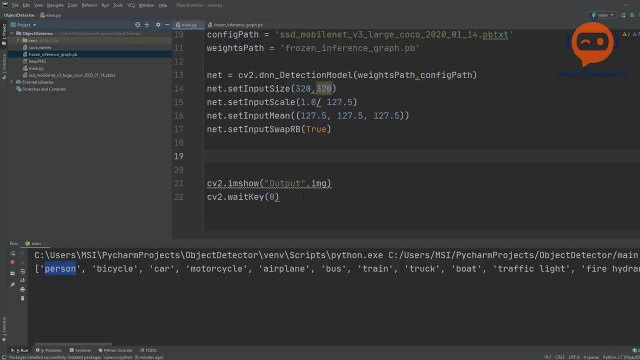 means. so here we are just going to write input swap rb and we will write this as true and the the idea behind this tutorial is that we should be able to get up and running object detector as fast as possible, without going into too much installations and too much formalities. so if you want to use it in a 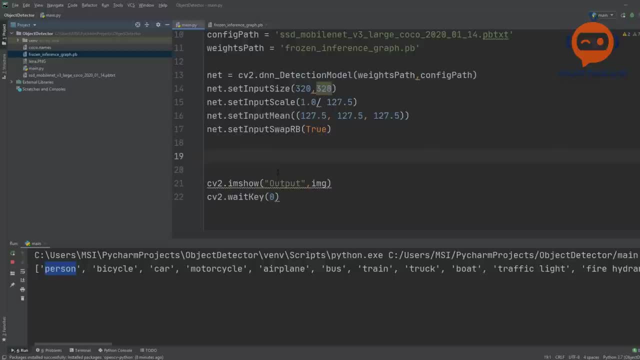 robot. if you want to use it in a self-driving car, you should be able to just use this small amount of code and just plug it in, and you should have object detection ready for you. so this is the main idea behind this tutorial. so again, uh, where were we? so we have done all of this. now what we need to do is we need to send. 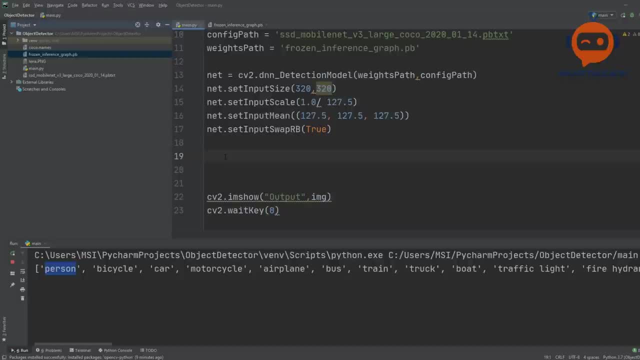 our image, to our model, and then it will give us the predictions. so we will write here class IDs and then we have the configuration, uh, the confidence, and then we have the bounding box. so we will write here: net dot detect, and we want to detect on this image. 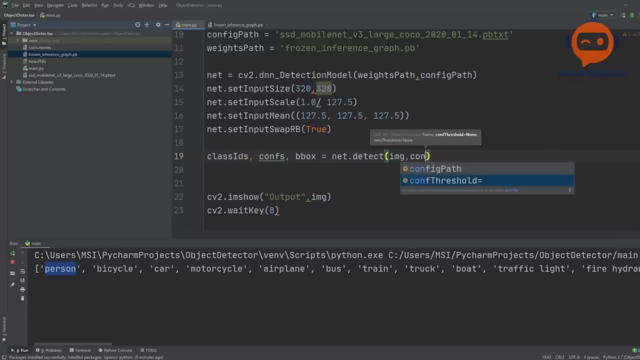 so the first thing we have to define is the uh confidence threshold. so at what point do we detect it as an actual op? so if it's sure that it's 50 an object, then we can say, okay, that is good enough for us. if it's lower than uh 50, then we will say that, okay, yeah, you should ignore that. so here we. 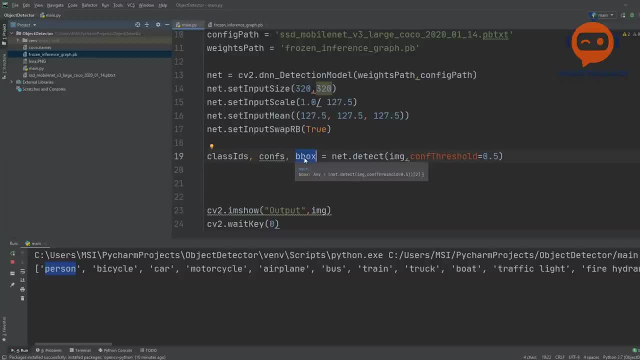 are simply getting our bounding box. from this bounding box information, we are going to uh create the rectangle on our objects and we can also write the name based on our class IDs. so we will see how we can do that. so that is good so far. what should we do next? okay, let's uh should we print this out? 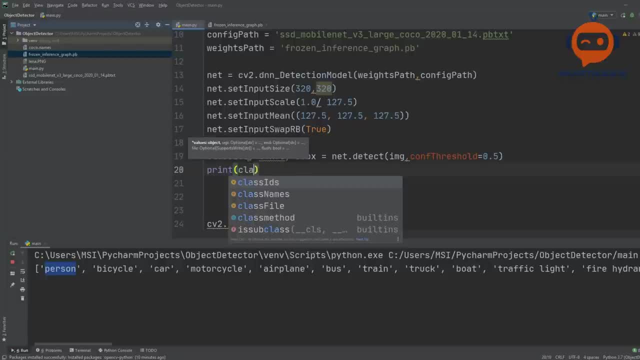 let's print this out. so let's print class ID and let's print the bounding box. so let's see what happens. and there we have it. so now it's giving us the class as ID number one and it is giving us this as the bounding box. so we have four values. we can use these values to create the rectangle. but here 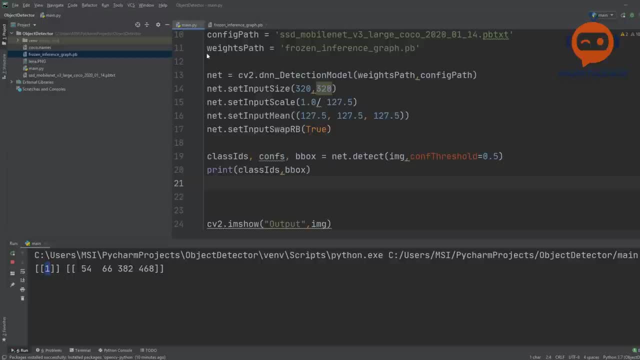 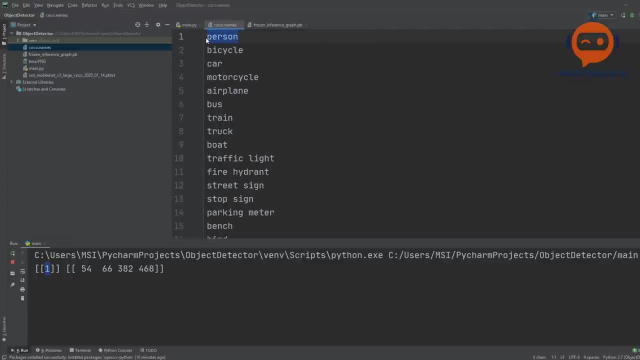 you can see, this is the interesting part. so it is giving that this is the first one, and if we go to our names now, this is indeed the first one which is person. but the thing is that if we look at the class names, uh, it starts from zero, not one. so when we are referring to it, we will have to 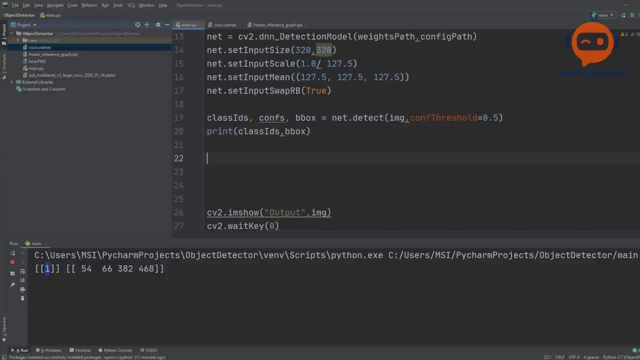 subtract, uh, one from this value. but that's not a big thing, we can do that, and so let's do this. we are going to. first we are going to write four class IDs and then, for confidence- confidence actually- we are talking about one specific ID. so however many IDs we have found, we are going to Loop through. 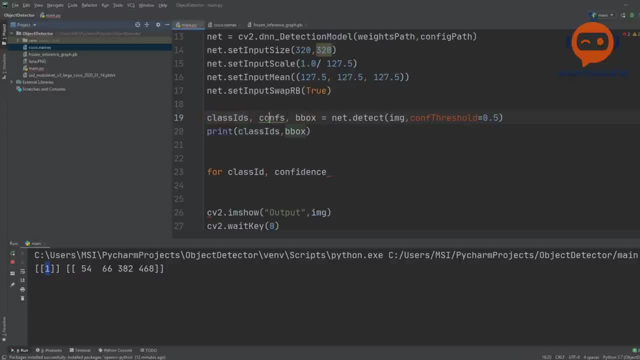 them. and now the thing is that we have three different variables or information that we want to Loop through. so we don't want to put three different four loops, we want to put one, just just one for Loop and we want to get all the information within that Loop. so to do that we can use the zip. 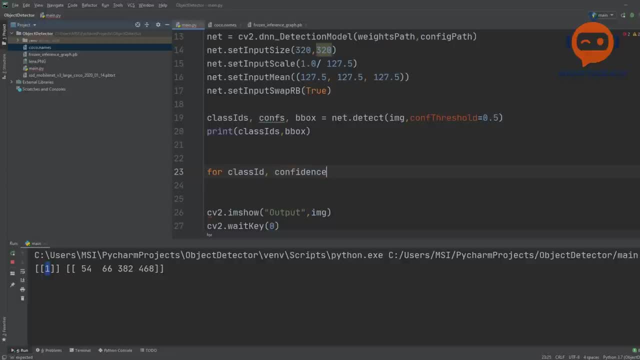 function. so here we have confidence, and then we are going to write box, then we will say in. so normally what we do is we say for uh, let's say class ID, ID in class IDs, right, so this is how you would normally write. now this is referring to 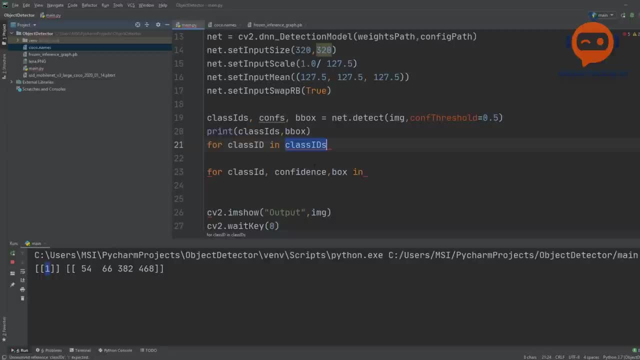 one, so, uh, one list, but now we have three different lists. so we have to use zip, so we will write here zip, and then we will write here class IDs and we have to flatten it, to use flatten, and then we have the confidence dot, again flatten, and then we have at the end the bounding box. so this is our for Loop and I can remove that. 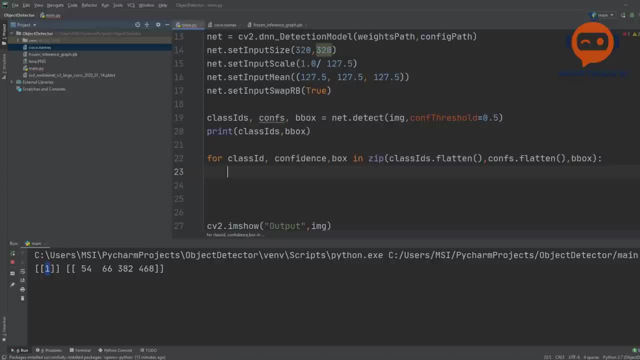 and then we are going to simply create a rectangle. so we will write here: cv2 dot rectangle. where is it rectangle? and then we will write image, and then we want to send in our bounding box and we just define the color of the bounding box. so color is basically: what is the color? let's put the color as zero, two, five, five and. 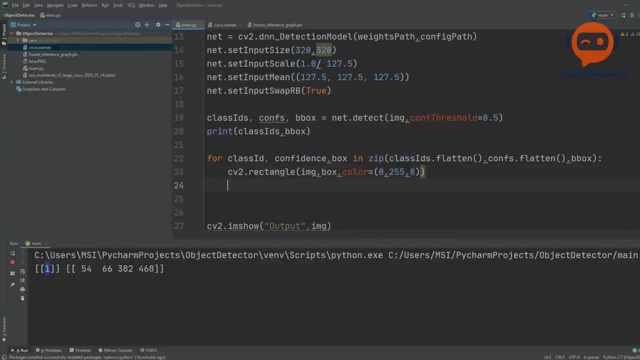 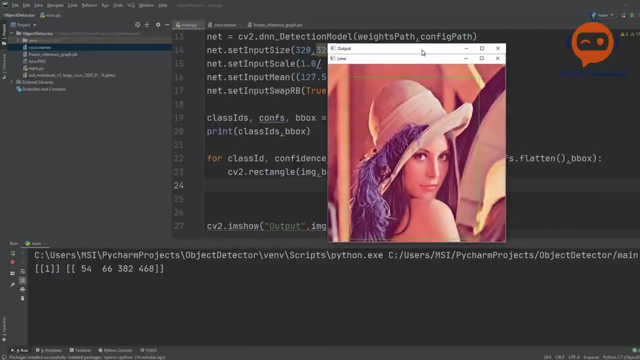 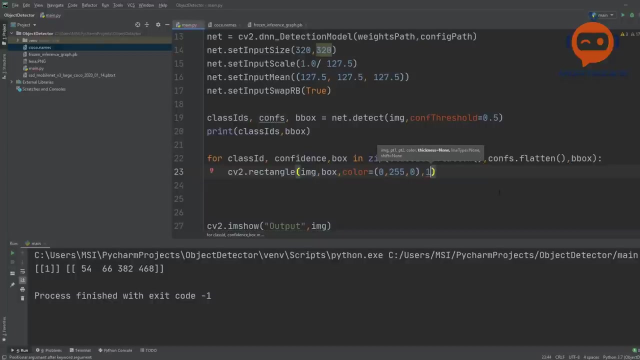 zero, so that will give us green. uh, yeah, that will give us green. so let's run this. and there we have it, excellent, but it's a little too thin, so let's just increase the thickness. uh, is it the next parameter? yes, it is, so we will write. let's say three. 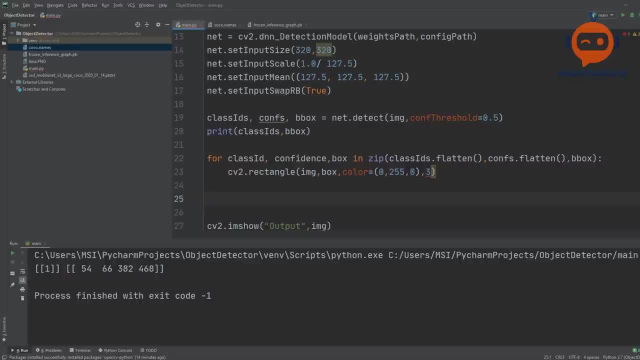 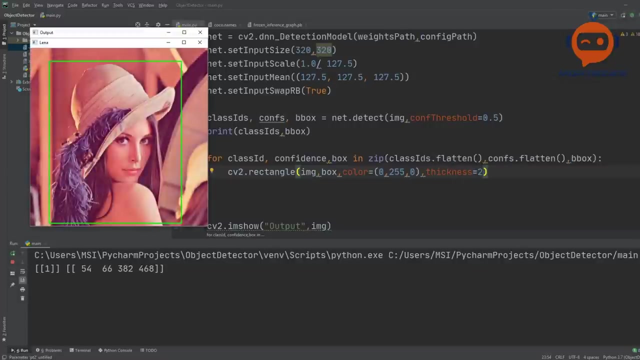 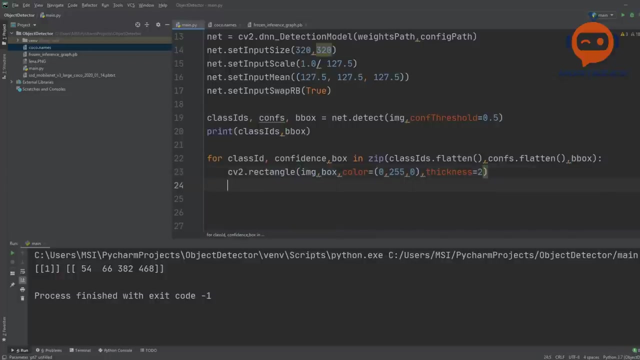 what happened? why is it another wait parameter? it's thickness. okay, let me write it down: thickness is equals to two, and there we have it. so now we can see that lina is being detected properly. so what we can do is we can actually write the name as well. so here we can write cv2.puttext. 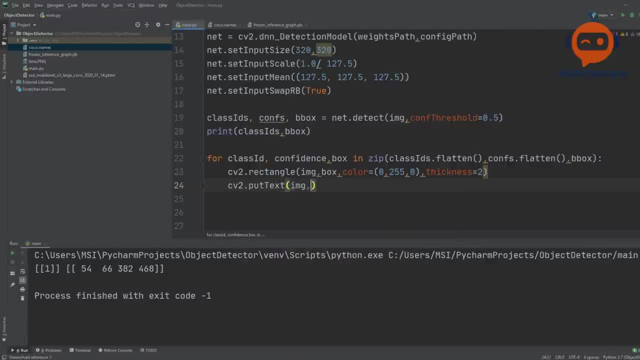 we want to put it on our image and then we want to write the name. so how do we get the name so we can write here class names and, as i mentioned before, we need to subtract the value. so whatever class id we have, we need to subtract one from it and then we will write the bounding box. 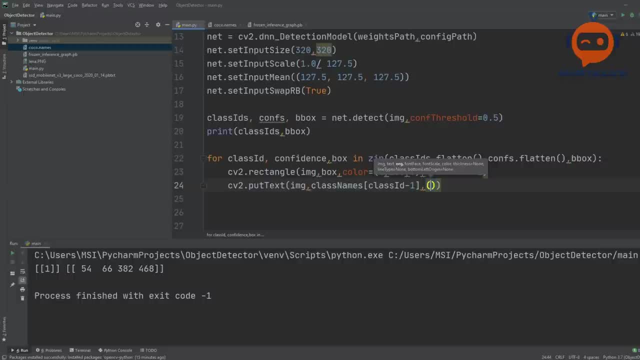 uh, not the bounding box, the points, the origin point of our text. so here we will use the box. so we want to get the x and y position, the origin position, and we are going to give- um, let's bring it down a little bit, so inside the box, okay, so we will. 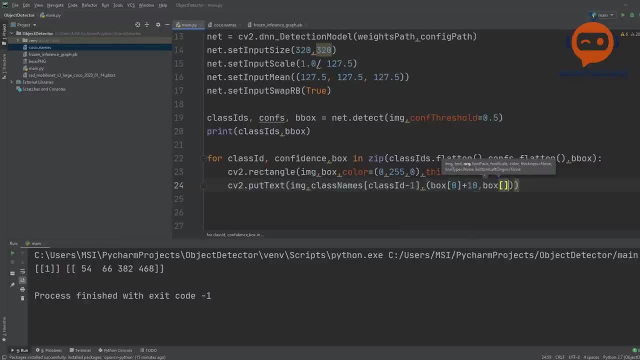 say, let's say plus 10, and we will say here: um, this one is, let's say, plus 30, so it comes down a little bit. and then we have to decide on a font. so let's say cv2- let me bring it down- cv2.font- let's pick any font, it doesn't matter. 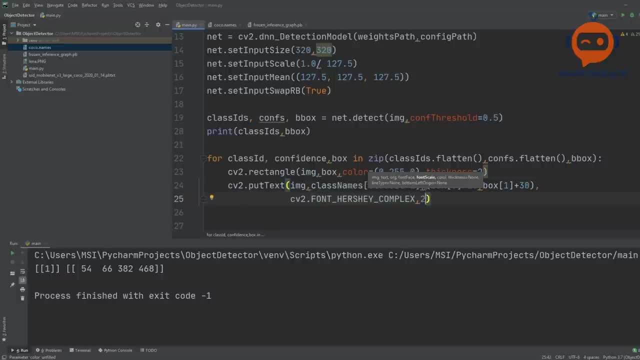 and what else do we have? we have scale. let's put scale as 2, and then we have the color. so color we can put as 255, or let's keep it green, so 0, 255 and 0, and the thickness we can put as 2. 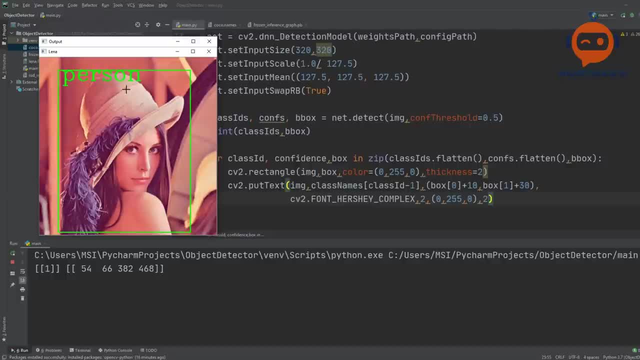 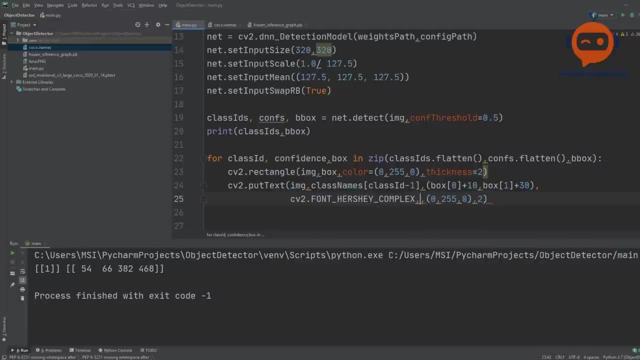 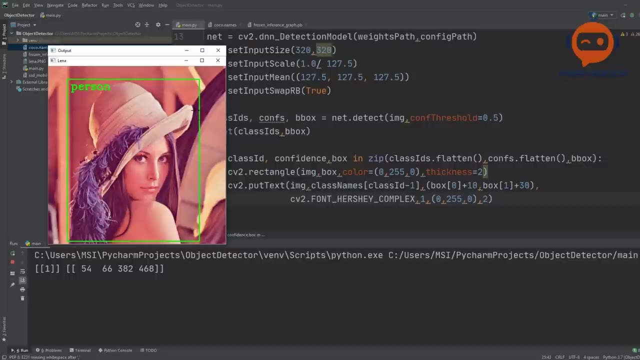 so i think the scale will be too big too. yeah, it's too big anyways, but we are getting, uh, the label as person, so the class we are getting properly. so let me just change that again and let's see: yes, so that looks good, so we have the person being detected. 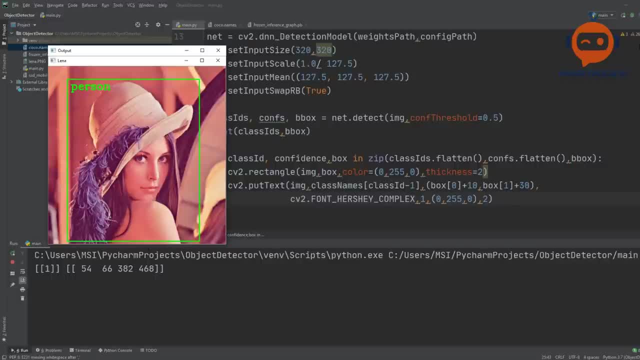 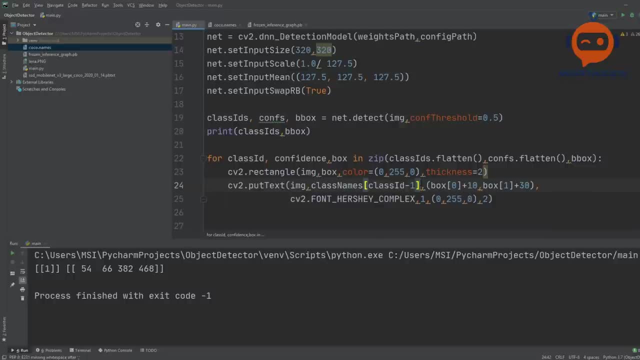 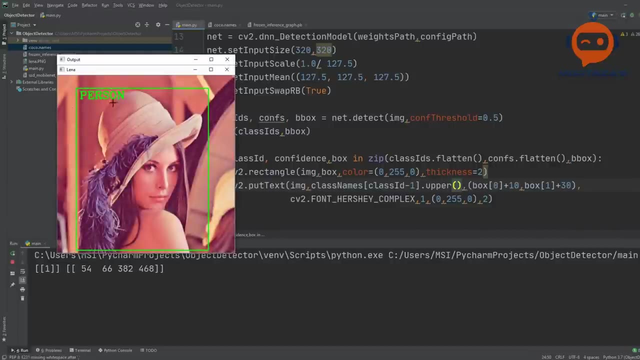 and we have the appropriate bounding box around it- excellent. so what else can we do? actually, this looks a little bit bad because i think it should be capital letters, so let's write upper here and let's run it again. yeah, that looks better. so we are detecting a person now. 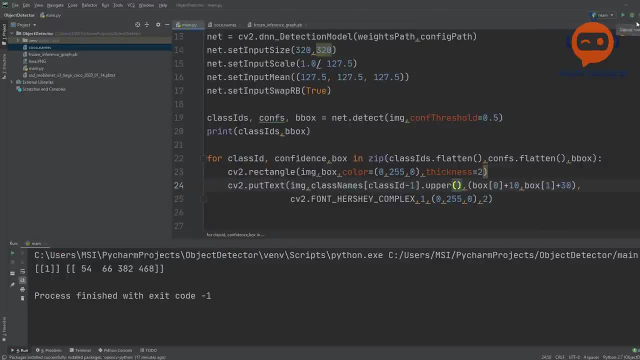 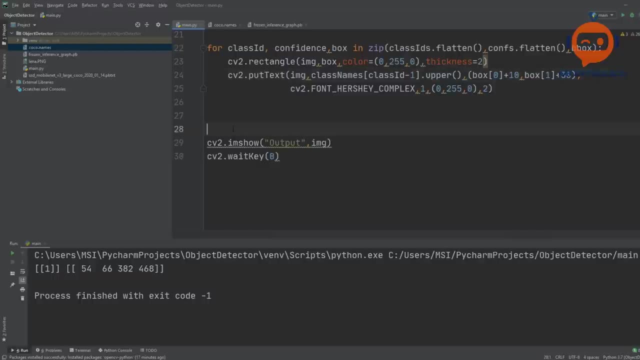 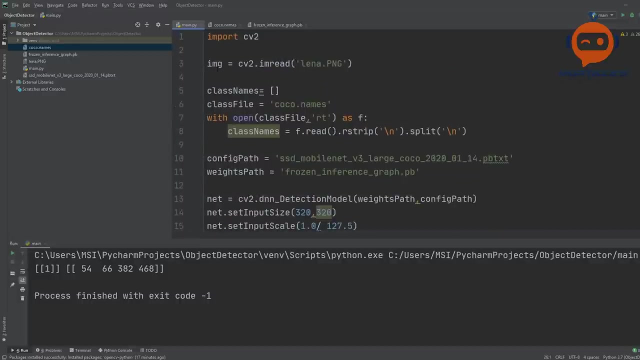 and we have the bounding box and everything is good. so what can we do next? um, yeah, okay. so now we will change this so that we can run it with an actual webcam rather than just an image. so we will remove this and instead of this, we are going to write here: 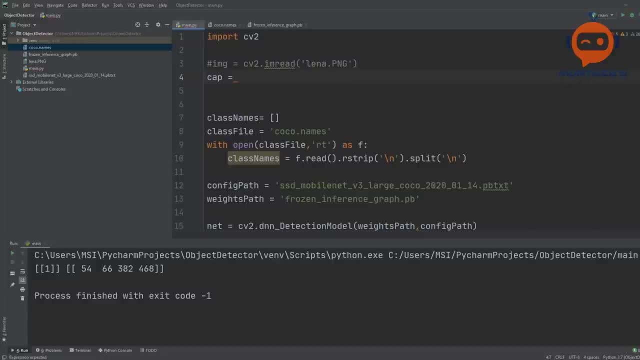 cap is equals to video capture. uh sorry, cv2 dots video capture, and then we will write here the the id of our camera. so in this case i will put zero and most probably it will not work because i use multiple cameras, so i will change it then if it doesn't work- so most probably it's going to be- 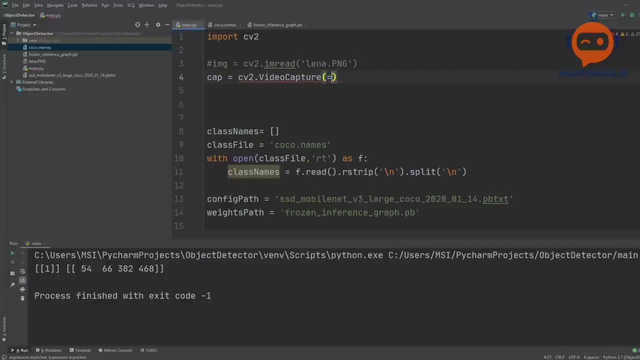 one, uh, actually, let's- let me just write one, because i know it's not going to work- um, and then we have to define. we can define, uh, certain parameters on how big our image is. so we can write here, um, let's say, cap, dot, set, and we have the three as the width, which is our prop id, and we can put it as: 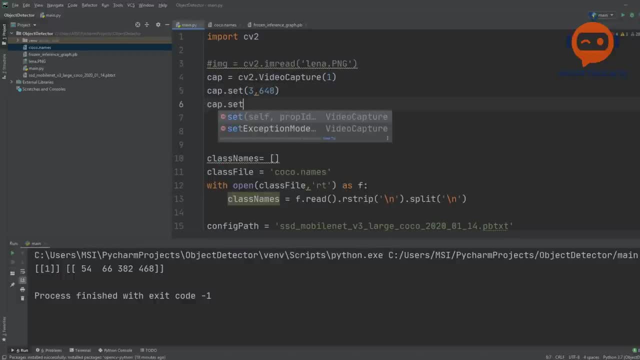 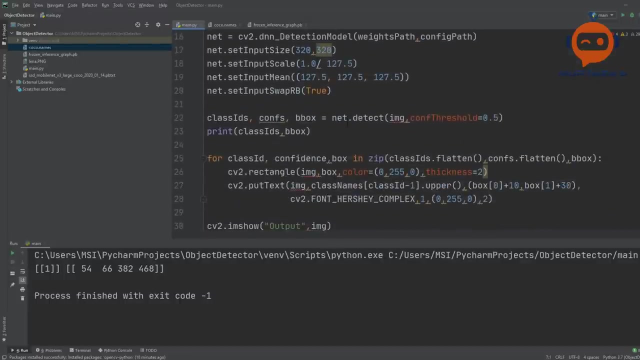 640. and then we have the cap dot set, we have prop id 4 and we can set it as, let's say, 480.. so again, that is not compulsory, but you can change that. and then which part are we not changing which does not need to be in the loop? 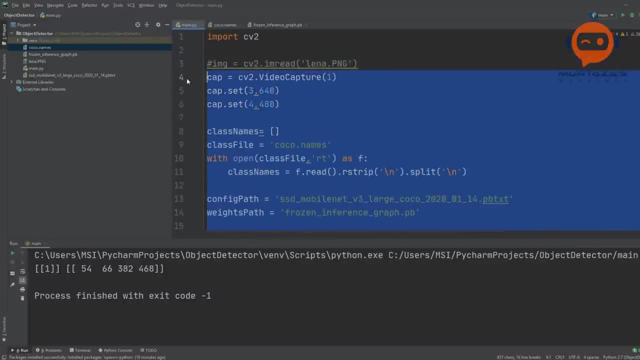 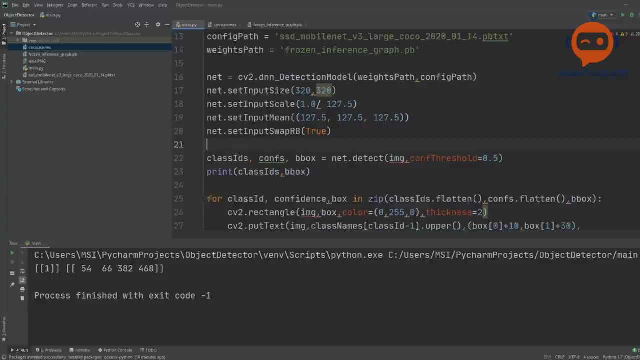 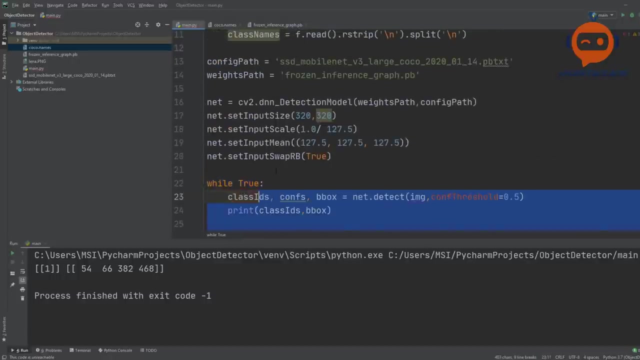 all of this is just setting right its initial part, so it does not need to be in the loop. starting from here, this needs to be in the loop, so we will write here while while true, and then all of this needs to be in the loop and this needs to be one, and we need to define our 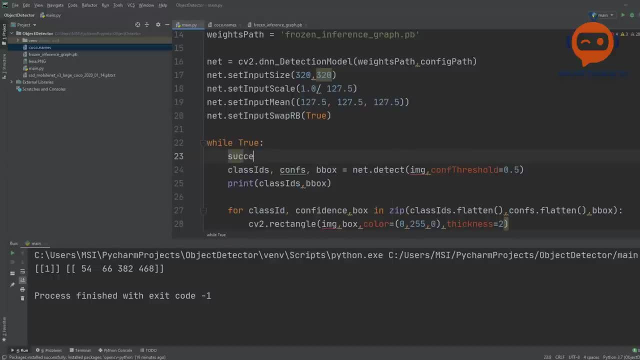 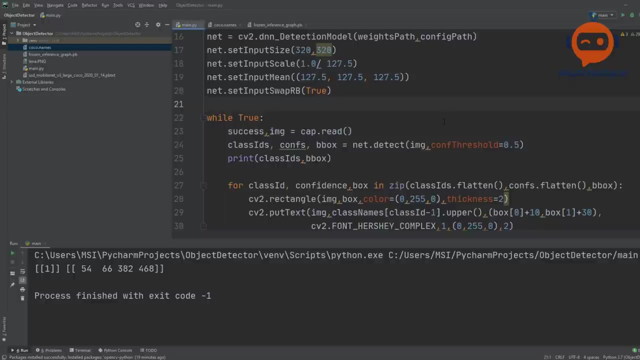 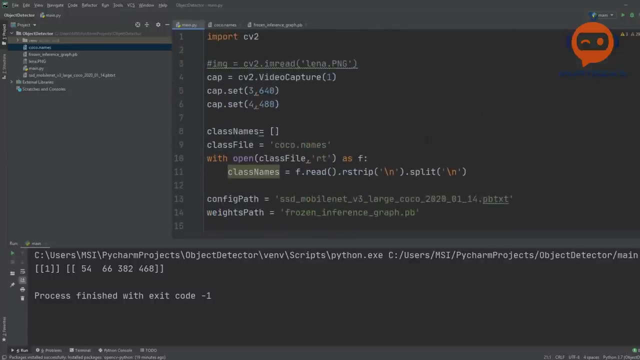 image. so the image basically is: we will write here: success and image is equals to cap dot read and this shall give us our image. and do i need to change anything else? well, so far it doesn't seem so okay, so let's run it and test it out. 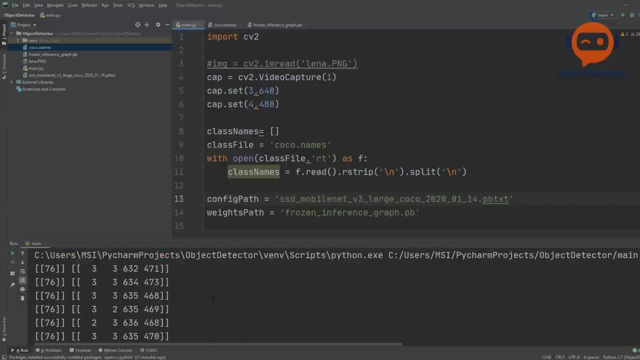 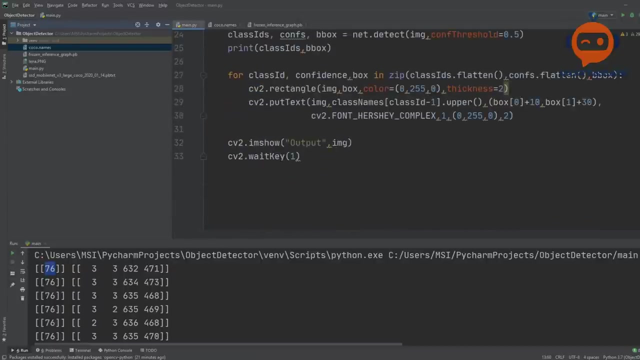 oh, so it showed keyboard and we can see this is 76. what is 76? 76 is keyboard. yes, so it is showing properly, but we ran into an error. why is that so? attribute other tuple object has no attribute flatten. okay, so what is happening is that we are getting when we are not getting anything. it's unable to process one of the lines. 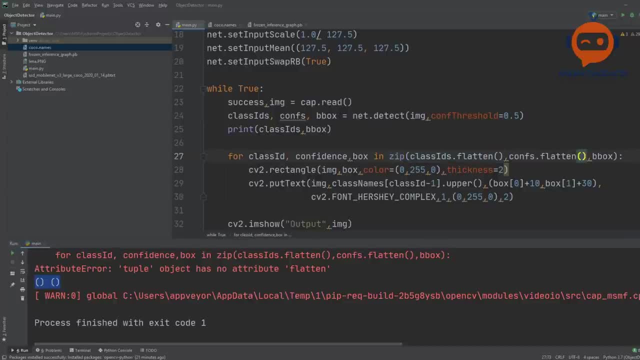 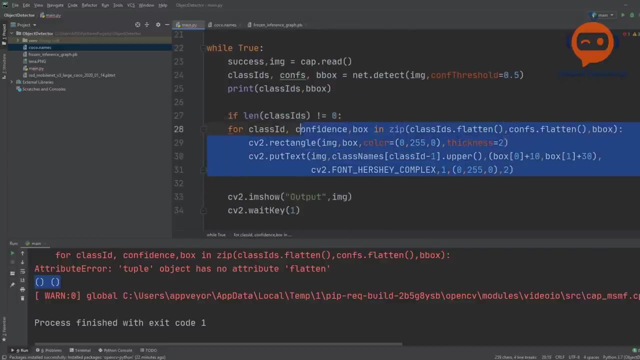 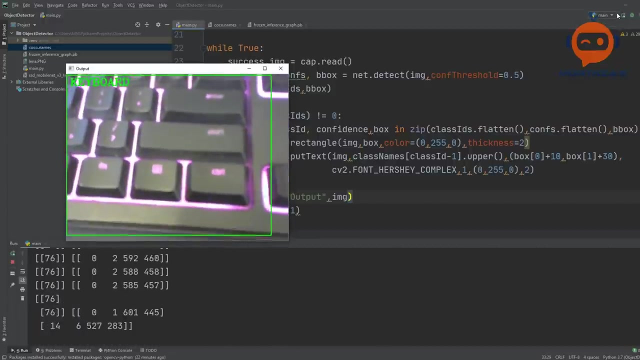 which is this over here. so what we have to do is we have to put here, we have to check before we go in- that the left mouse button in the dialog. so we know here that i am going to be here just being a cursor and let's put row equal to zero and the left mouse button is the whether. next time when i come to theним Э. discarded without a reason. so i can't take back what was on this list over here on this page. of course class id is not, because class id is usually flying in a rosy wet calendar. so we can do that by writing if the length of any of our lists over here so we can write, for example, instructionspeak and something detected. it is not empty. so we can do that by writing if the length of any of our lists over here so we can write the class id is not equals to zero. so that should work as. 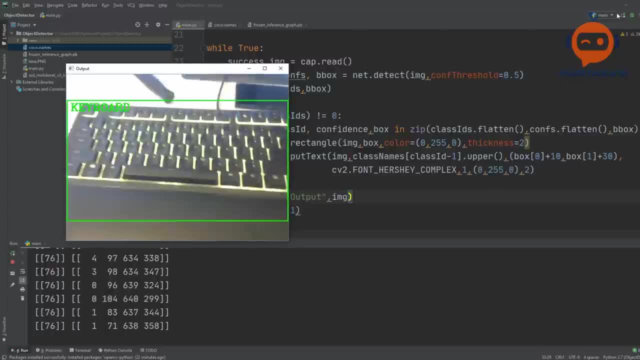 so this Wご時 رضیه صي력 keos' gear, if this time out of this maca is not going out, so that should work. have my keyboard here and you can see that it's detecting very well. then I have my monitor. it's. 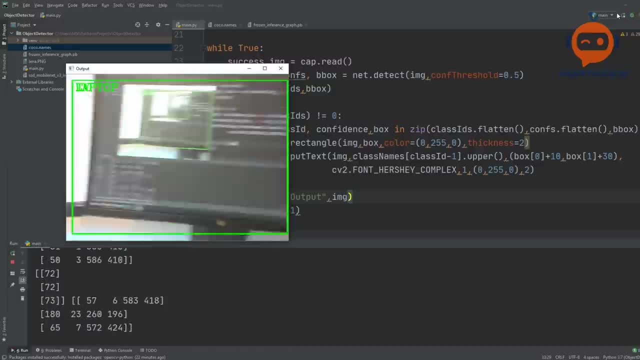 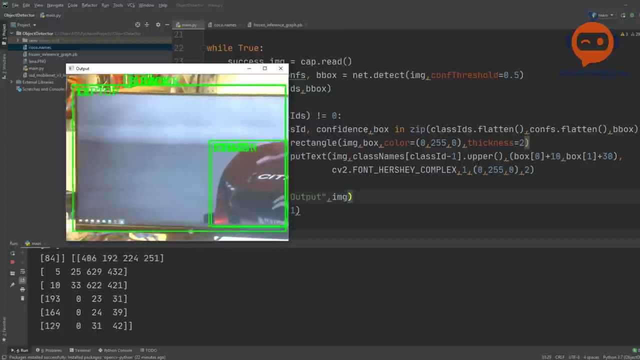 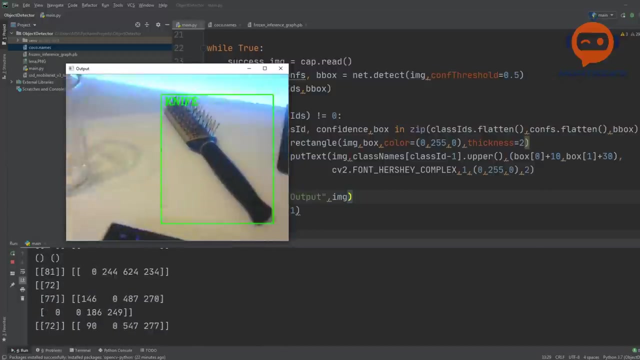 saying laptop or tv. it's a little bit confused between those two and if I do that here, you can see here it's again saying laptop or tv and let's try some other objects. so we have the cup and then we have another cup. we have what is that? toothbrush? uh, not so accurate, but close enough. 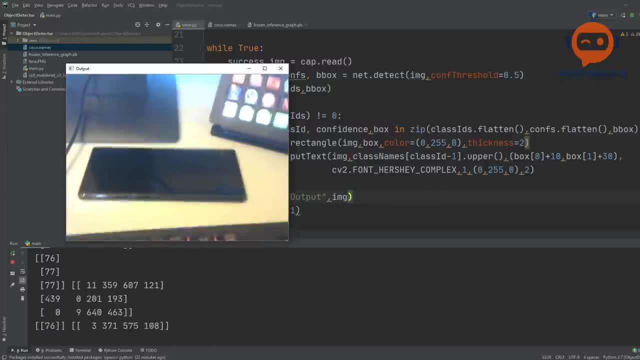 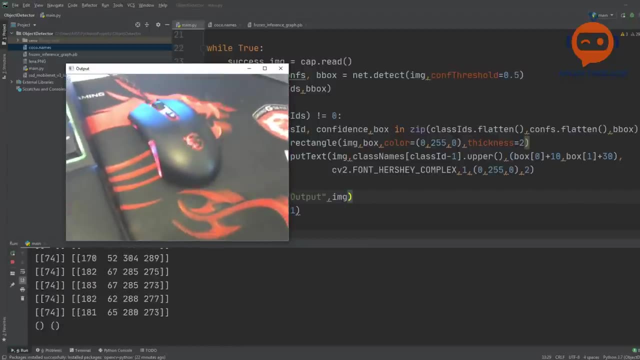 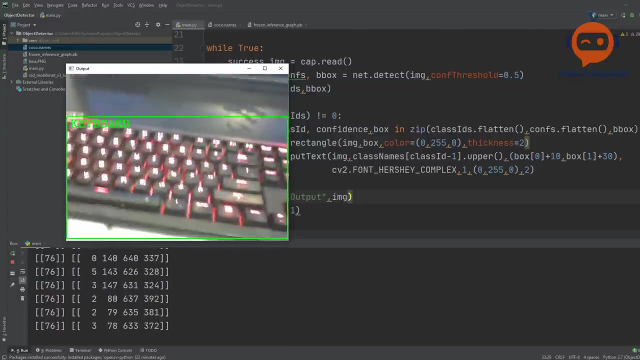 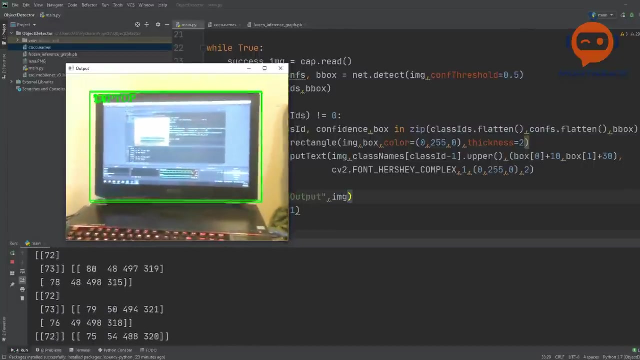 it's still a brush, but then we have, uh, the cell phone. yeah, we have kind of a laptop written here here. we have a mouse, that is good. let me check my laptop. yeah, in the laptop it says keyboard and let me show you here. so here it says tv, maybe laptop now. so it's a little bit overlapping, but it seems to be good. 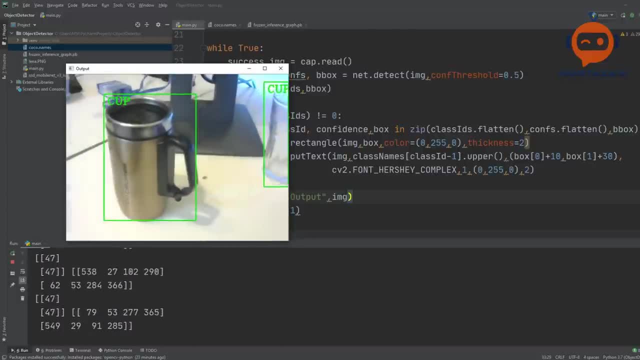 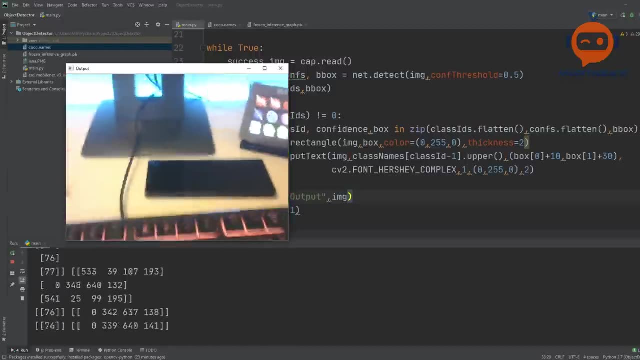 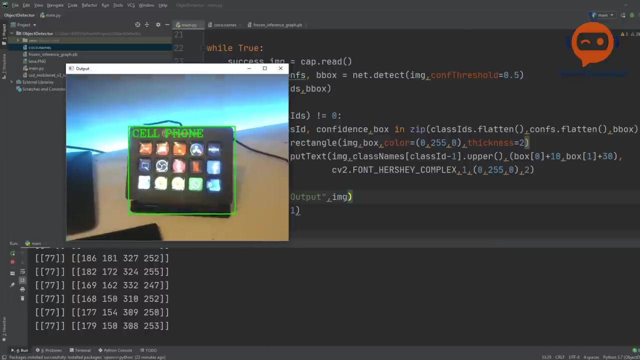 so all of these are being detected quite well and, as you can see, this is real time, almost real time, and I can move this around. yeah, this, I don't expect it to work properly. this is a stream deck. I wouldn't expect it to work properly. I would expect it to work properly. 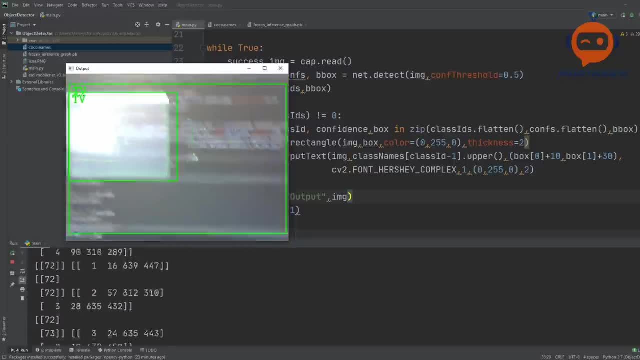 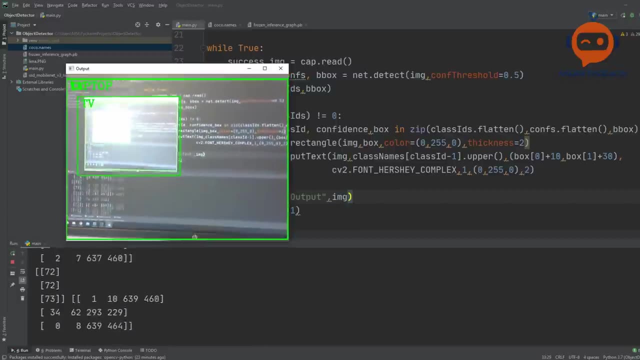 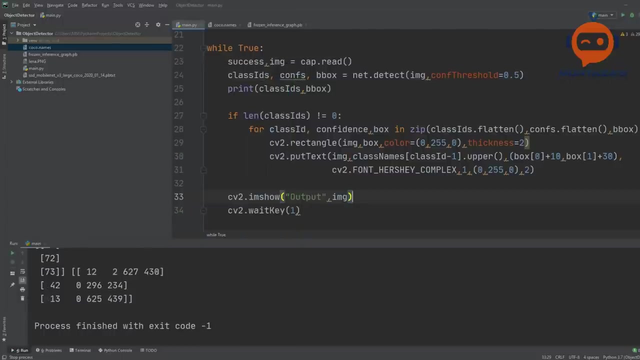 wouldn't expect it to know what that is anyways, but the good thing is we are able to detect. uh, again, it's not the best accuracy, but you are able to detect with a good amount of speed and a good amount of accuracy, so the balance is quite good. so what can we do next? uh, now, the only thing that 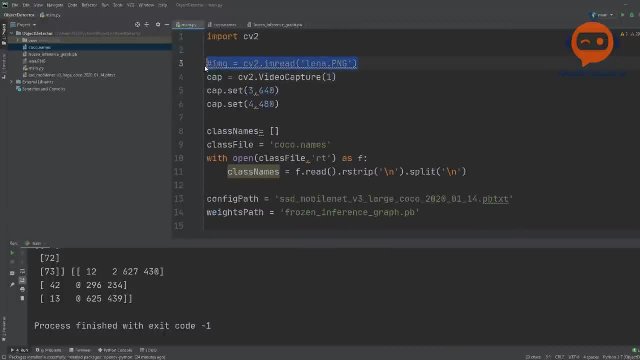 we can do here which remains is to actually put our threshold at the top so that if we wanted to change the threshold, we can add it up here. so here we can write that our uh threshold value is equals to this, and then we can write here that this is our threshold. 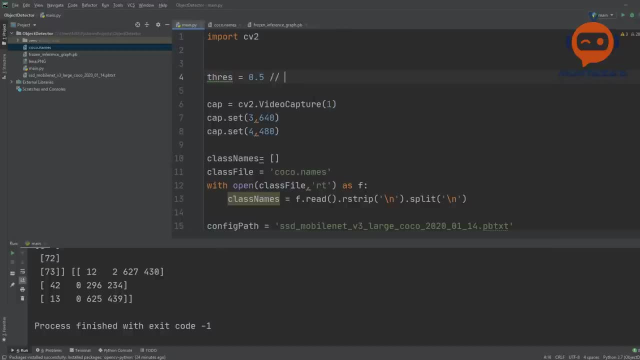 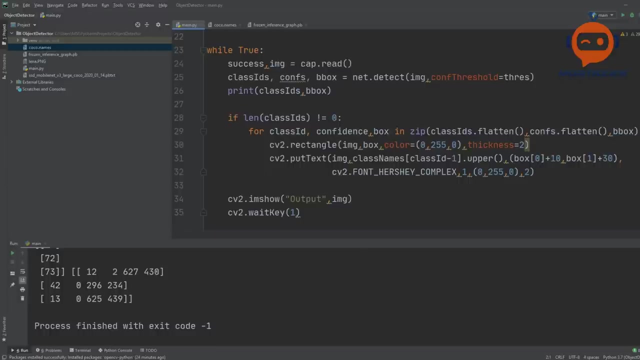 so we can write here: threshold to detect objects, okay, and we can also write the confidence values as well. so if we wanted that, we can simply put another text and we can write it here and the instead of the class name, we are going to write the confidence. 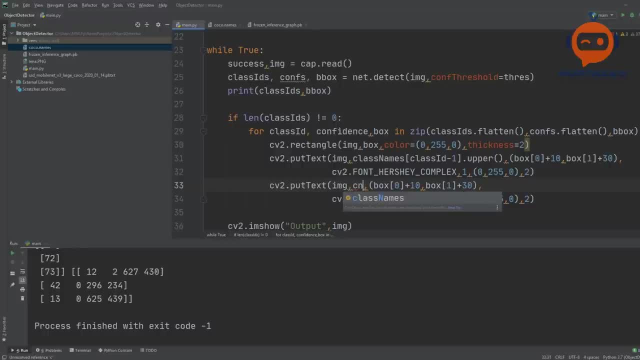 value, so we will write here. what did we write? confidence, so we wrote confidence, so we will write here: confidence. and should we bring it down or forward it forward? so let's put 50 and see how it works. okay and okay. so there's an error. okay, i think we need to check first: what kind of value are we? 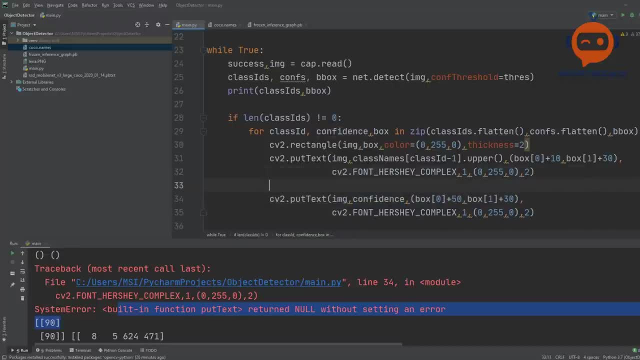 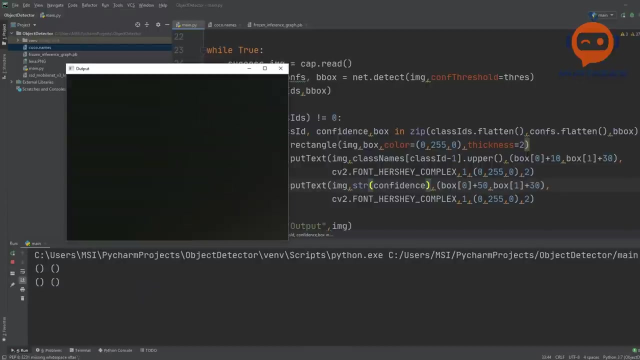 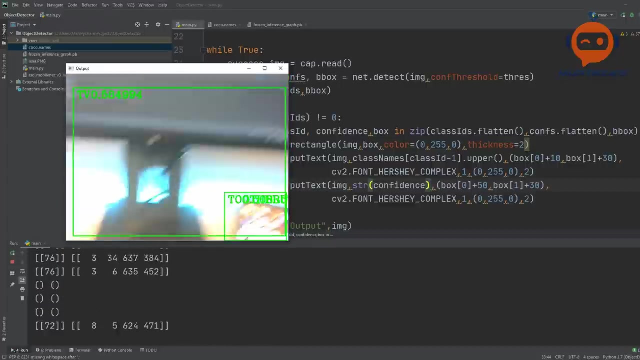 getting in confidence because it doesn't seem to be able to write it down. oh, it's a. oh, my bad, it's a value i forgot, so we have to change it to string. uh, my bad, we have to change that to string and let's write. and there we have it. so now it looks really bad because it's overlapping and whatnot. 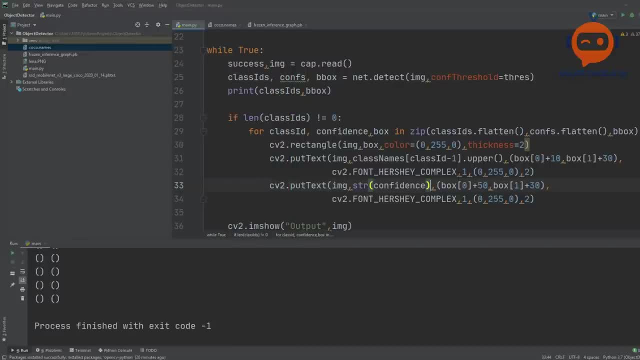 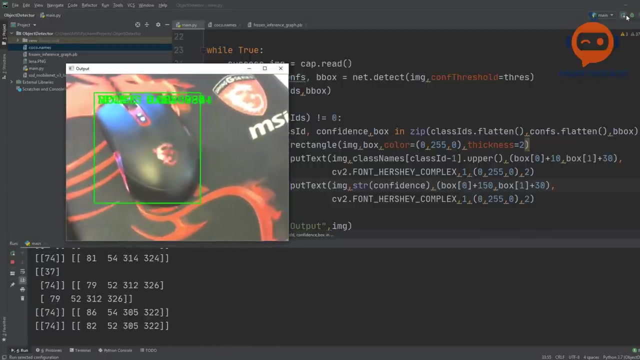 okay. so what we can do is we can bring it further and we can write here, let's say 150. maybe that will work. so if i have the mouse here and it's telling me that it's 0.6 percent, 0.5 percent, sure that it's a mouse. 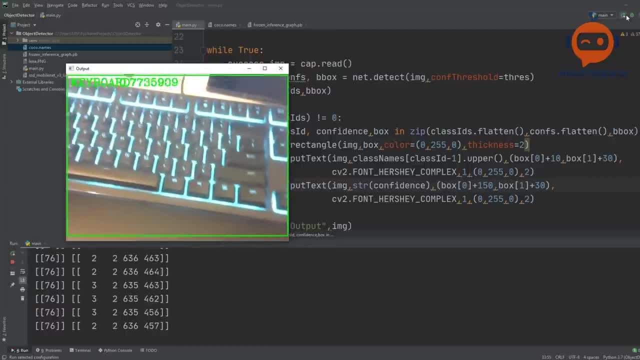 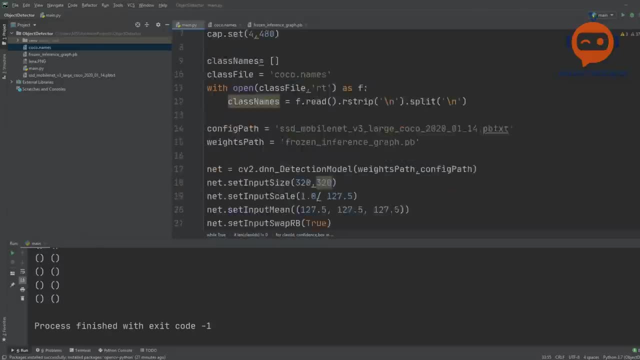 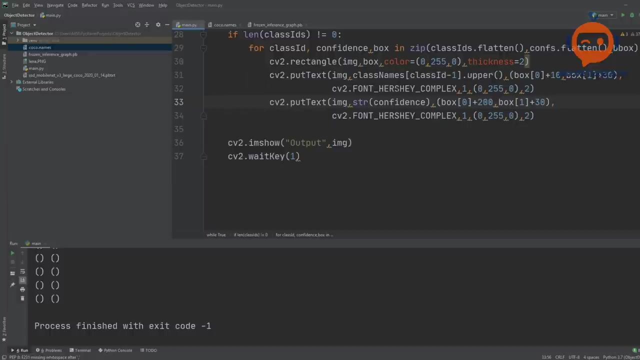 and it's fluctuating quite a bit. and here we have the keyboard and okay, so the value does not seem to be not good. what we can do is we can put 200 here and we can put here that we want to multiply this 500 and we want to round this off, so round, and we will write here where is the round. 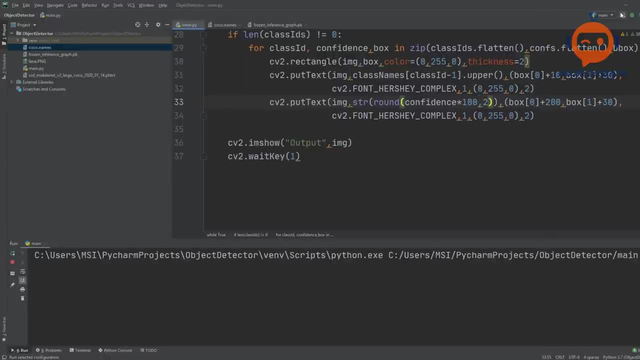 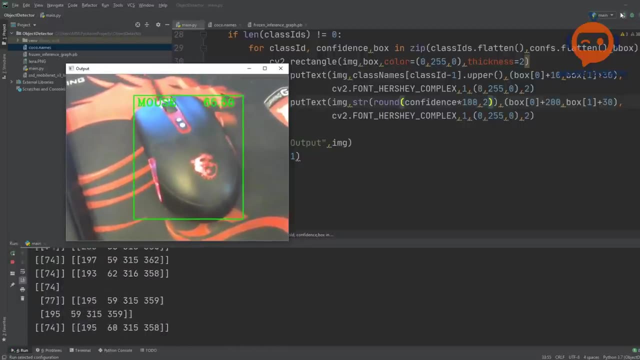 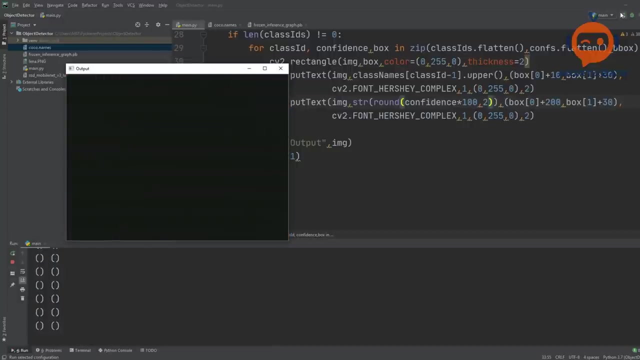 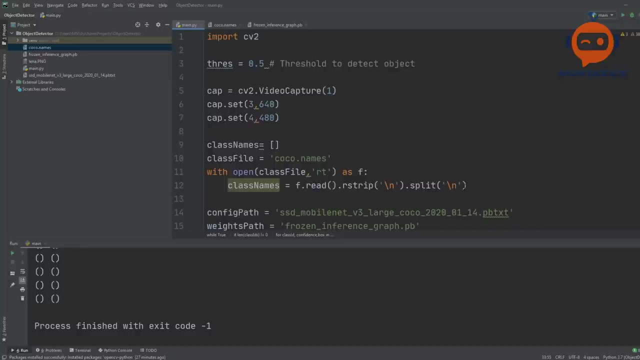 okay, so we're right here. 2 and let's see. yeah, so now it's more visible, so you can see mouse is 67, 67, 66, something like that percent. so that is good. so this is it for today's video. i hope you have learned something new. 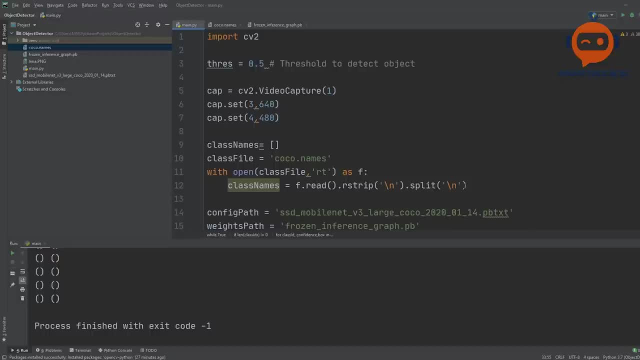 if you like the video, give it a thumbs up and i will see you in the next one.